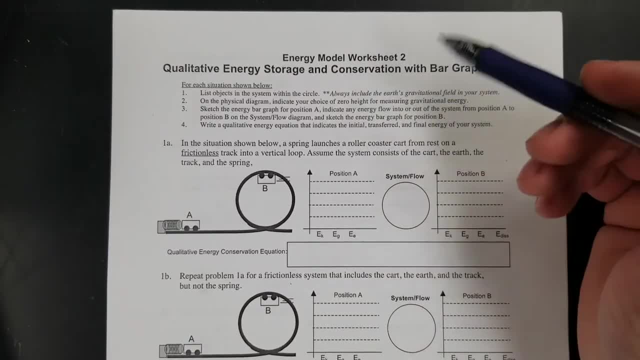 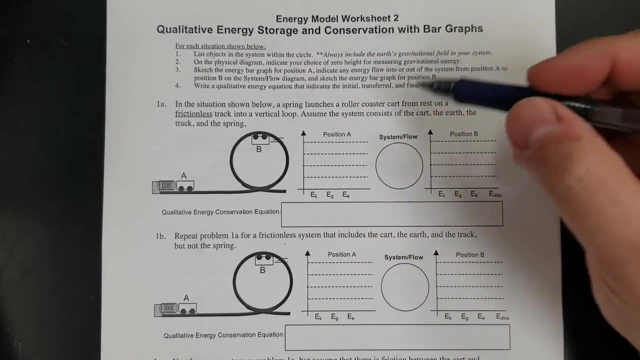 Okay, so let's solve a few examples of these energy problems. So what we're doing in all of these problems is you're practicing writing down what the system is and then looking at what's coming in and out of the system and then drawing a bar chart that shows how the energy is before. 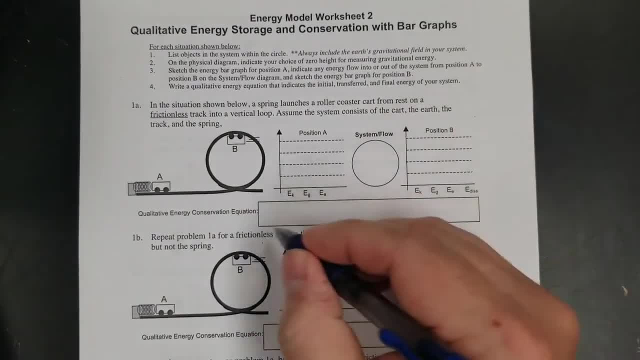 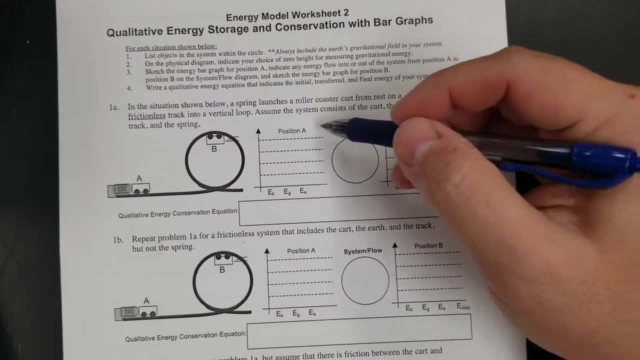 and after right, The different types of energy, And then you're writing an equation that you can use to solve for something, right? Not solving anything, just writing the equation. Okay, so let's start with number one. This is like a really basic example: Spring launches a road. 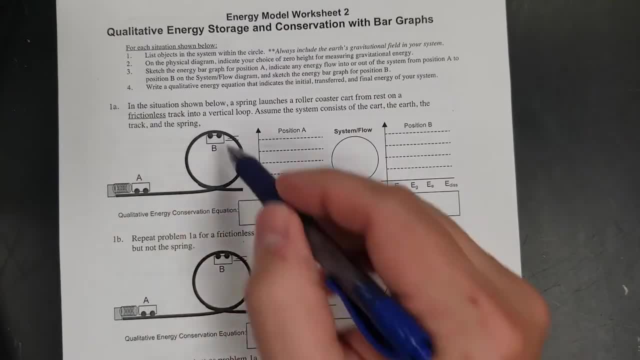 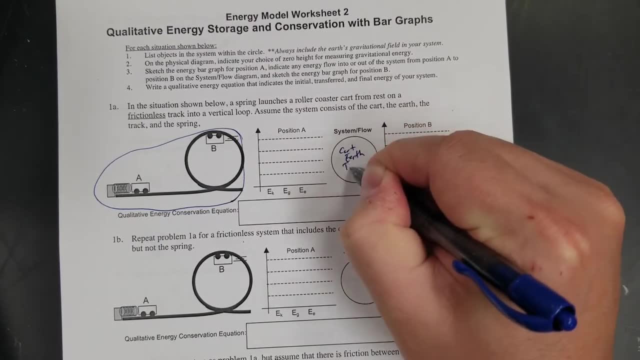 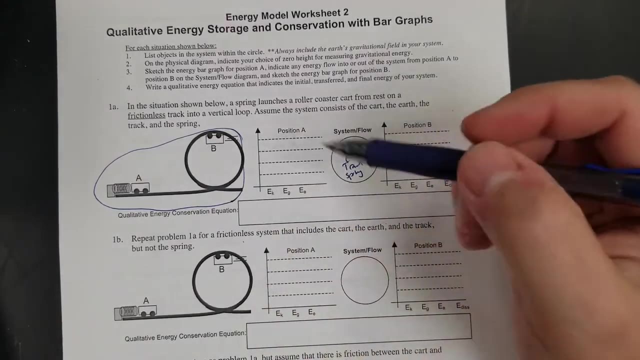 closer from rest. Assume the system, the cart, the earth, the track and the spring- right. So cart earth, track spring. Everything is in my system, right. So cart earth, track spring. Okay, so let's do the graph first. So what type of energy does it start with? Okay, so it's not. 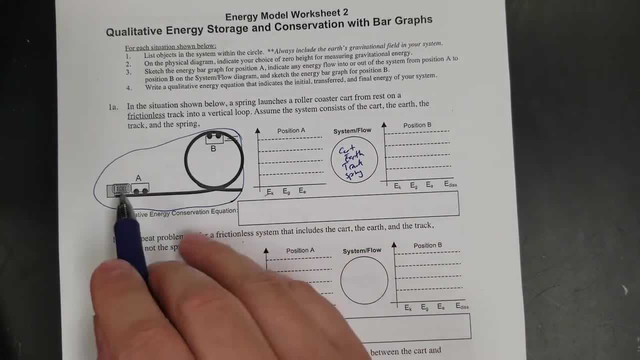 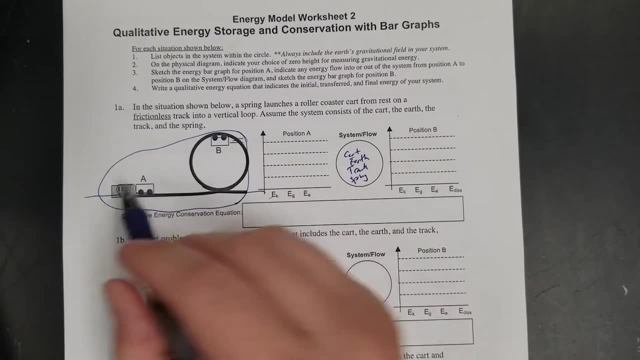 moving. so there's no kinetic, It hasn't gone anywhere. I'm going to call this zero, right? So there's no height, so there's no gravitational potential. Okay, so it's not moving, so there's. So there's elastic, because that spring is scrunched up. 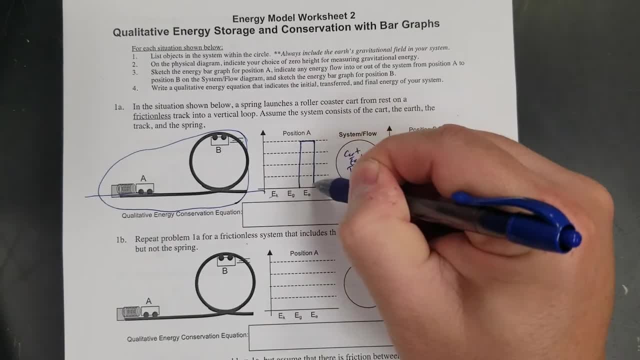 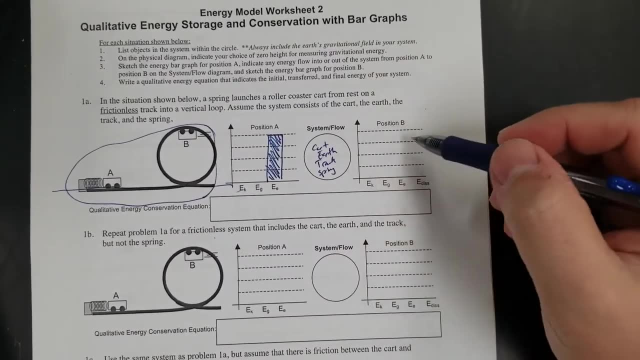 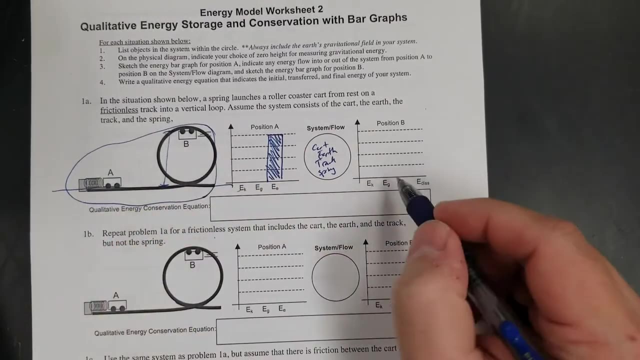 So I'm just going to make up, call it four bars. So that's my elastic potential at the beginning And then afterwards. position B: now it's moving right And it's higher up. So the spring is let go, so there's no elastic. 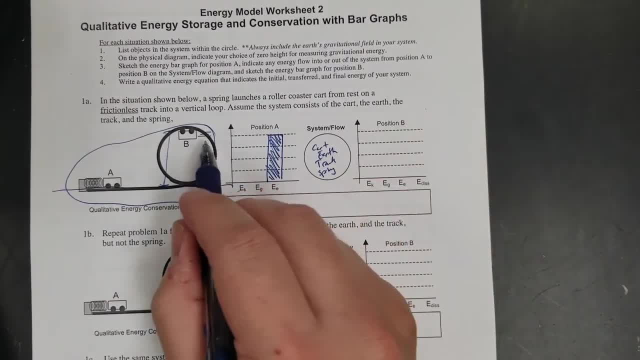 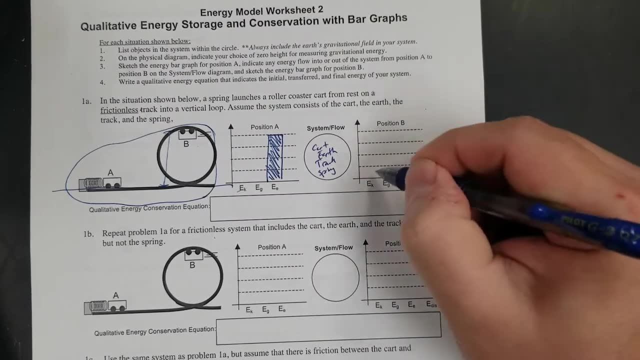 Gravitational? yes, there is gravitational And it's also moving. so there is kinetic right. So there's no friction, right? Frictionless? Okay, good, So there's no heat. So I'm just going to say two bars and two bars right. 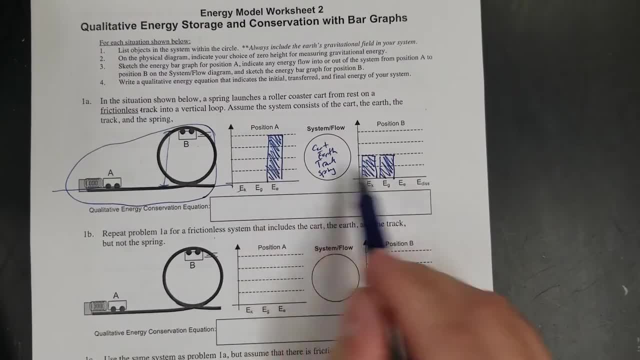 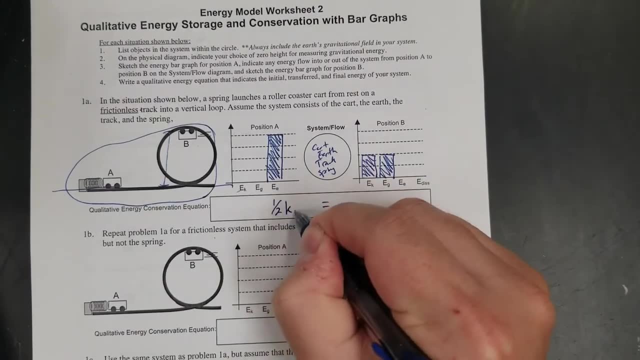 So I had four bars here. now I've got two bars and two bars, So four equals four. Okay, so let's write my equation. So there's elastic, So one half KX squared, And there's, on this side, there's kinetic and gravitational. 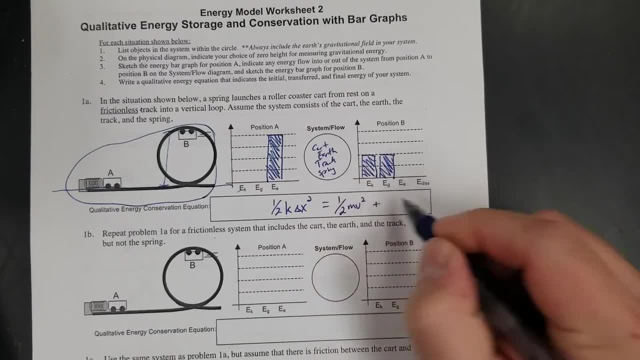 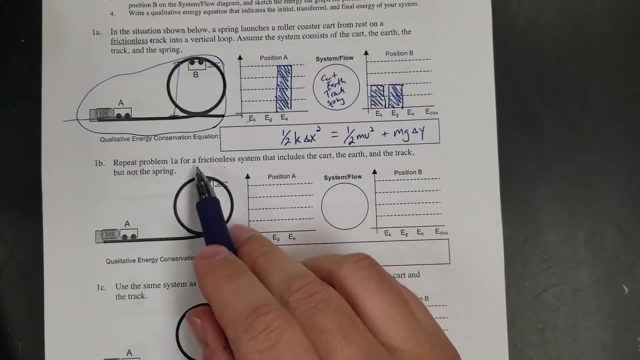 So kinetic is one half Okay, And MV squared plus gravitational is MG, delta, Y, Okay, All right. So second example: Frictionless system still Okay. So there's no heat Cart earth track, but not the spring. 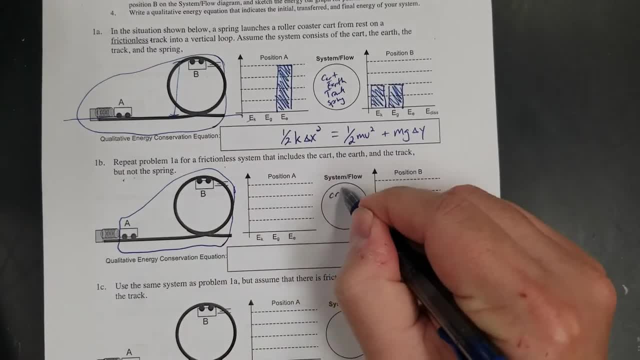 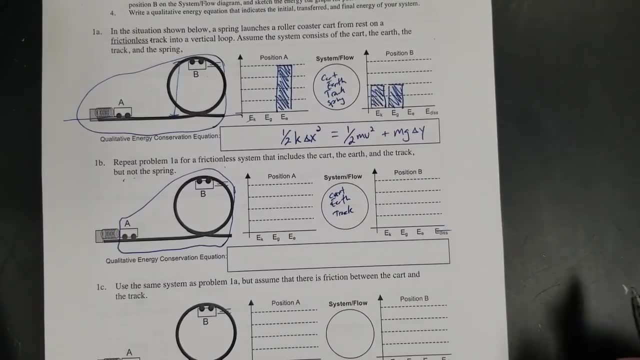 Okay, So my system is this: So cart earth track, No spring. I can't even spell, Okay, Well, so at the end it doesn't change, But at the beginning there's no spring, Right? So at the end I'm going to stick with my four bars, two and two. 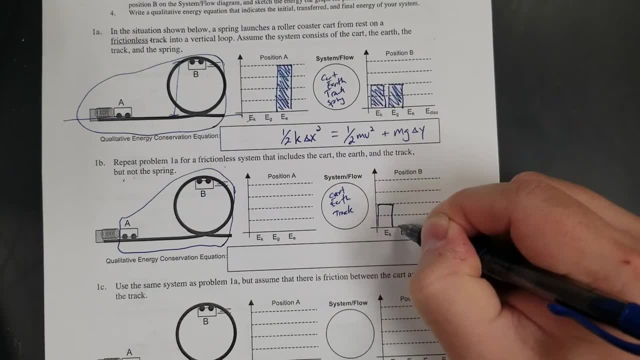 Right, But okay. So where did this energy come from? Well, it had to come from work, Right? So I'm going to represent that, saying work came into the system, Right? So here's my system: The spring is outside. 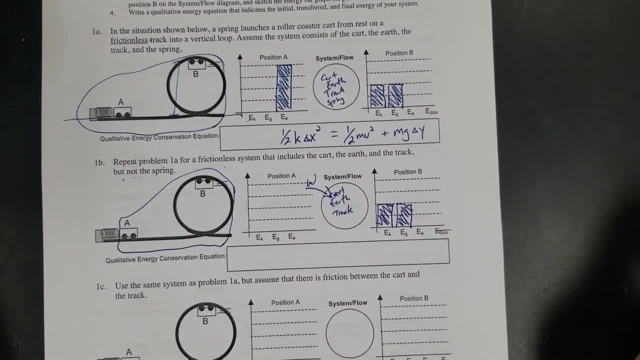 So it's putting energy in in the form of work. So my equation is going to be: work equals Right. There's no kinetic, There's no gravitational. It's the same as this one, except I just took the spring out of the system. 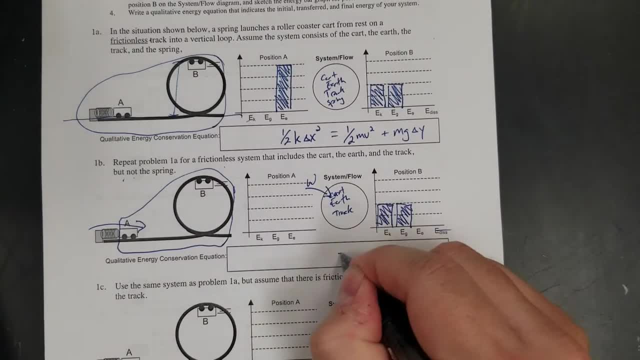 So one half MV squared, Okay. So there's no kinetic. There's no gravitational. It's the same as this one, except I just took the spring out of the system. So one half MV squared, Okay. So there's no kinetic. 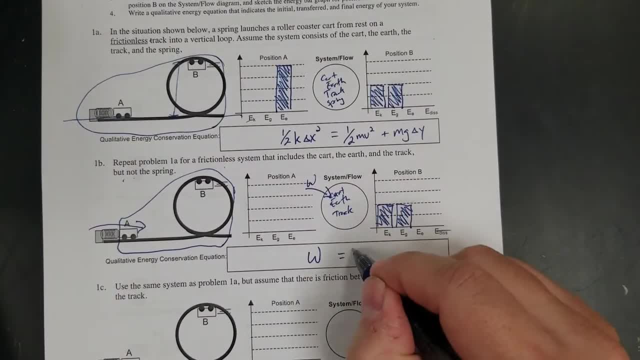 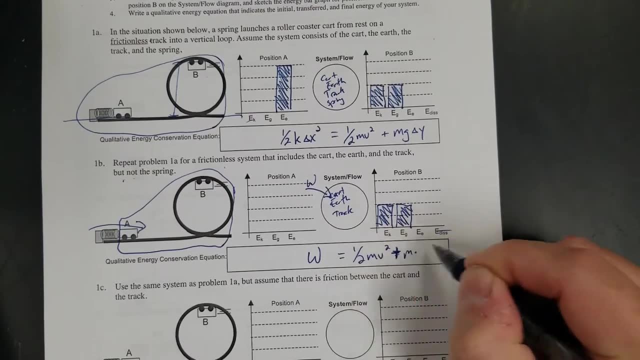 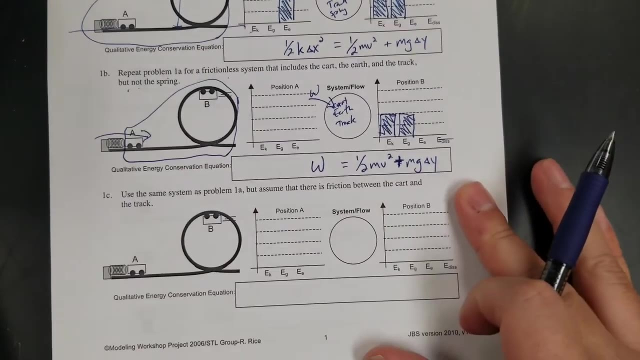 There's no gravitational. It's the same as this one, except I just took the spring out of the system. So one half MV squared equals no plus M, G, Delta, Y Right. So work equals the kinetic energy plus the gravitational potential. Okay, 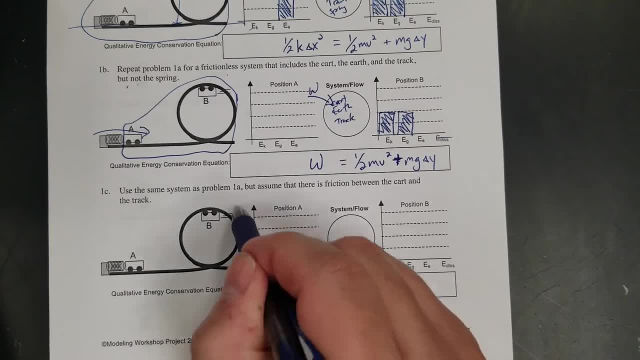 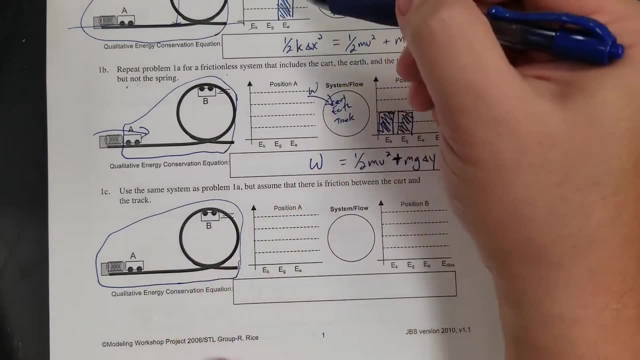 So same system as problem one. So now same system. That means everything's in the system. Now there's friction between the cart and the track. Okay, So I know I'm going to do the same thing. right, Because it says it's the same as one. 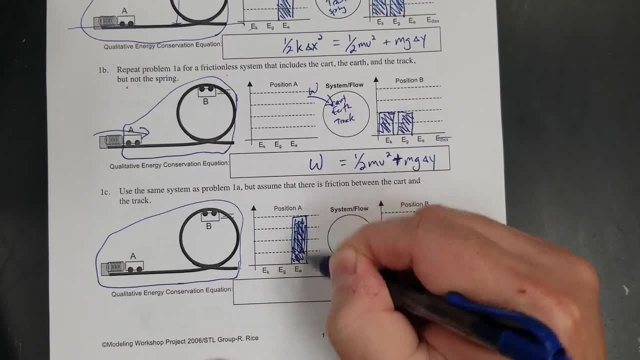 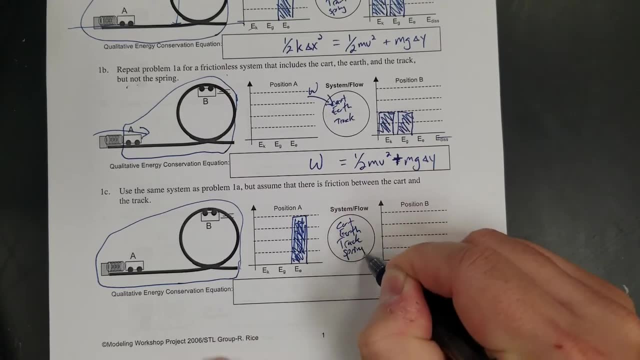 So I'll start with four bars. right, I'm just making up four bars, It doesn't matter what you start with. So cart earth, track, spring and then afterwards. now I have friction right. So if there's friction, there's going to be heat. 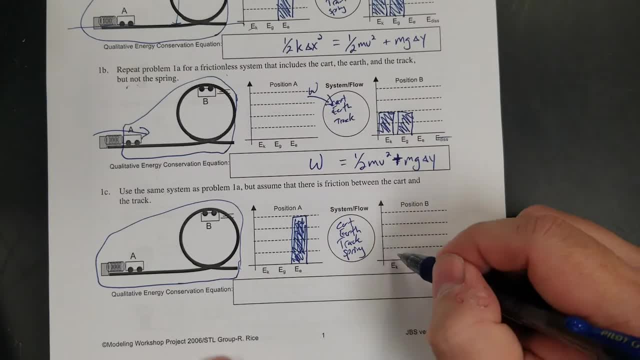 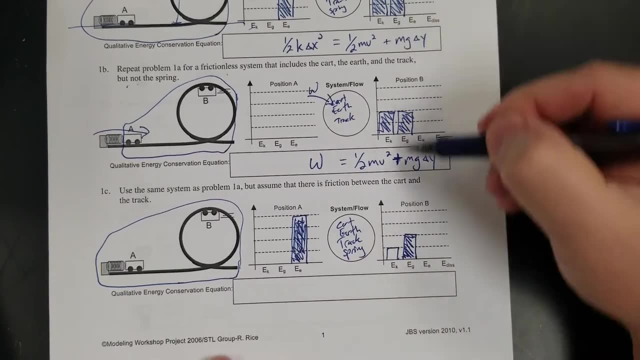 So let's say it comes out of the kinetic because it'll be going slower. So the gravitational: I'll still say there's two, right, Because it's still at the same height as my one. before I had two bars here, so I'll put two gravitational bars here. 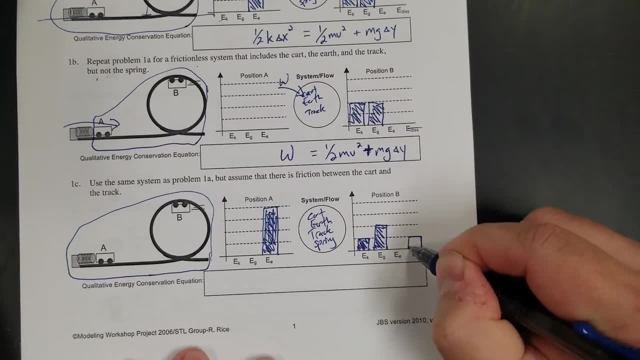 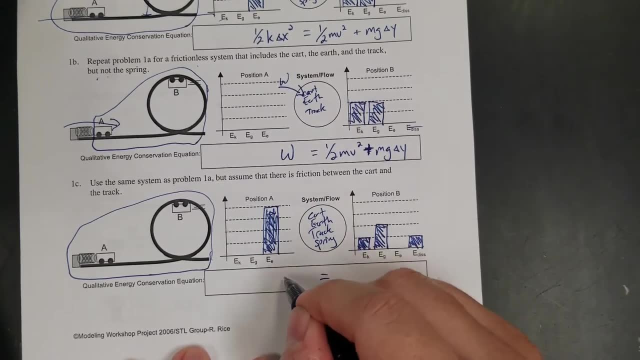 But now I'm only going to have one for kinetic and one for heat, So it's going to be going slower here because that friction has taken away some of the energy. So write my equation: half K X squared equals half MV squared plus M G, Delta, Y plus the heat. 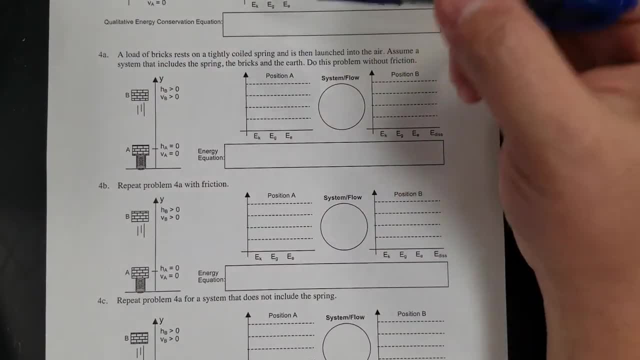 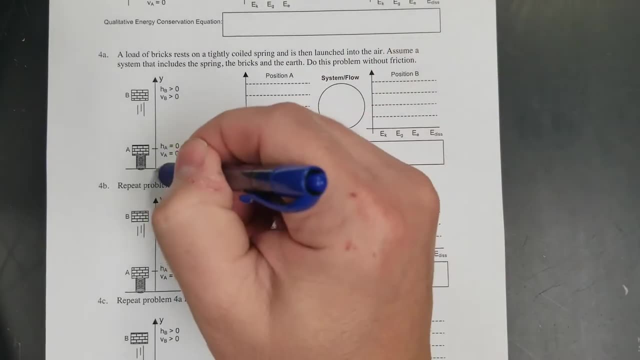 There we go, Okay, So let's try another one. So load of bricks is rested on a tightly coiled spring is launched in the air Soon. the system includes the spring, the bricks and the earth. So spring, bricks, earth. 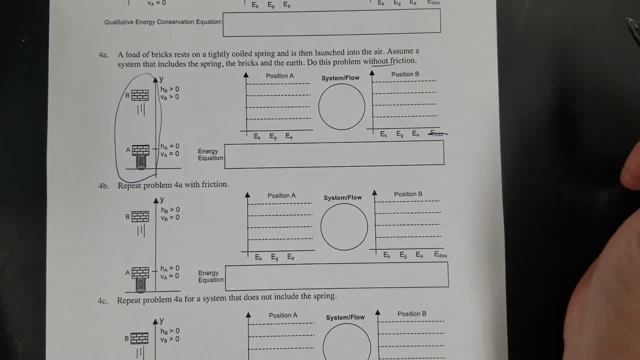 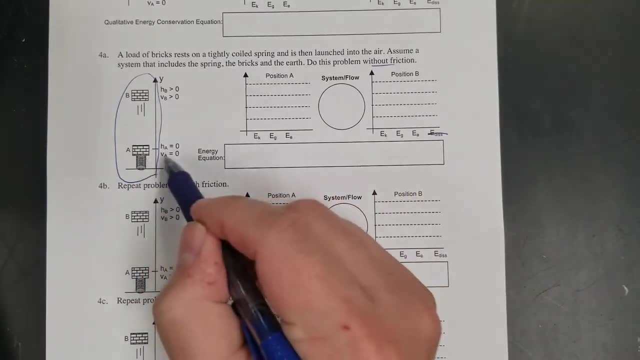 Do the problem without friction. So there's no heat, All right. So if it starts coiled up and it says the height is zero, so there's no gravitational right, Because it's calling this zero. So it's all elastic stored in the spring. 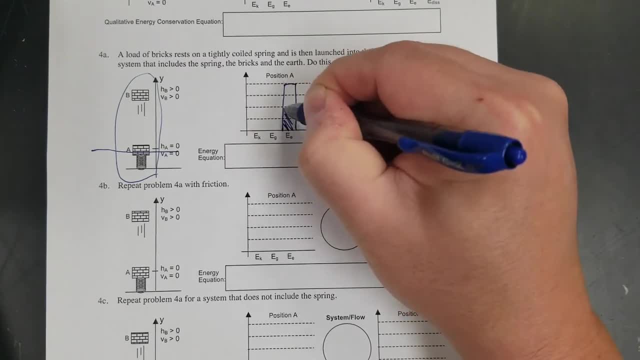 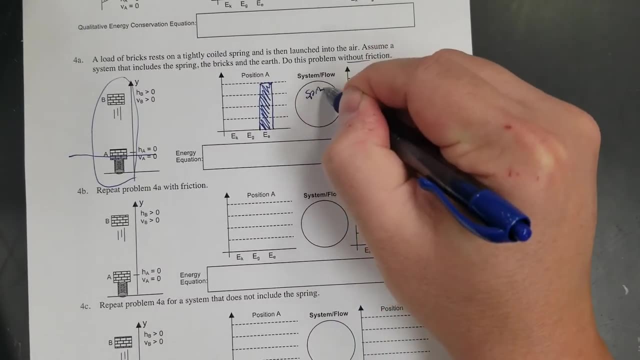 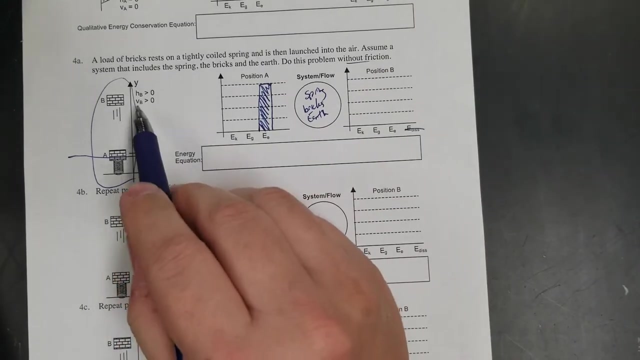 So I'll just Okay. So I'll start with an even number, I'll start with four, right? So what is it? spring bricks, earth. And then at position B, it's above the ground, right, So it's got gravitational. 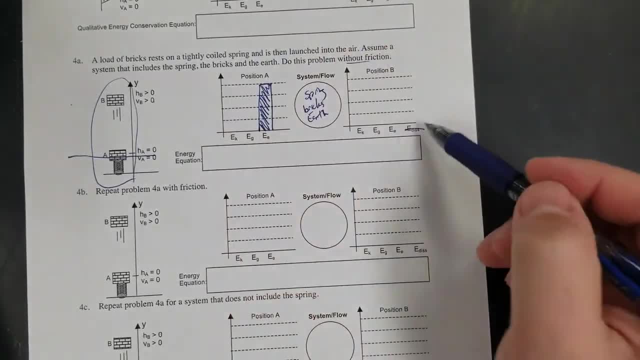 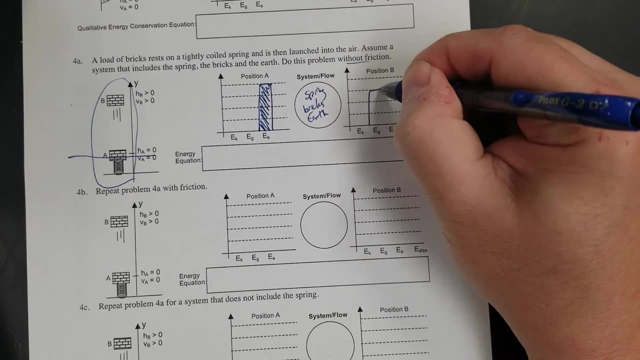 It's moving, so it's got kinetic and it's frictionless. So there's none of that. And the spring has already let go, so there's no elastic. So it's just between kinetic and gravitational. So I'm going to say three gravitational and one kinetic, because it's high up right. 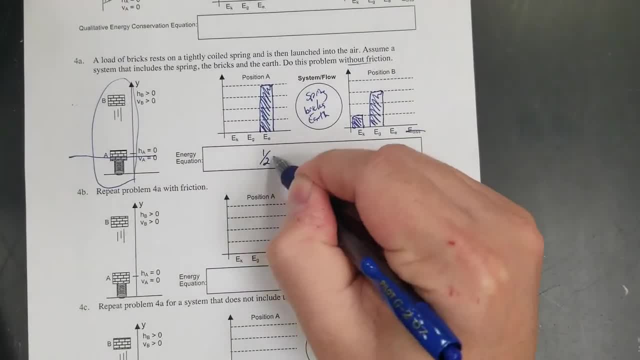 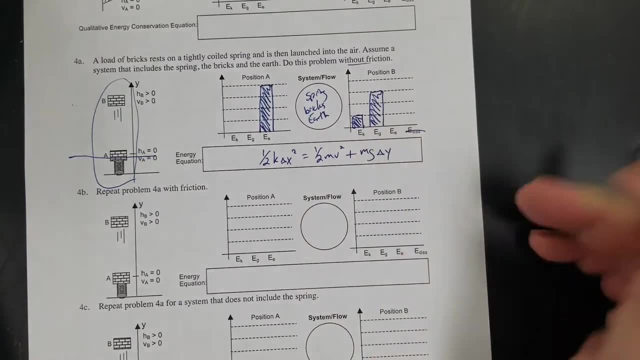 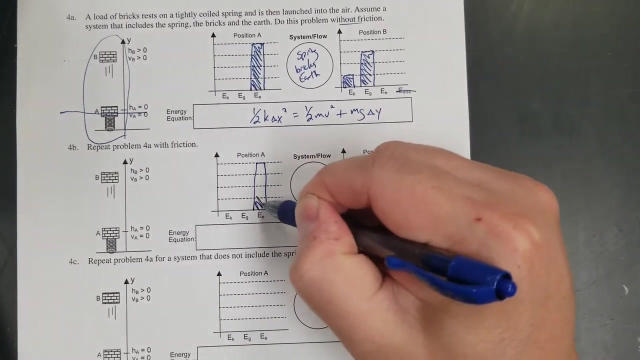 As long as it adds up. So one half kx squared equals one half mv squared, plus mg delta y. Okay, Repeat it with friction. So I'll do the same thing, right? And then spring bricks, earth, All right. 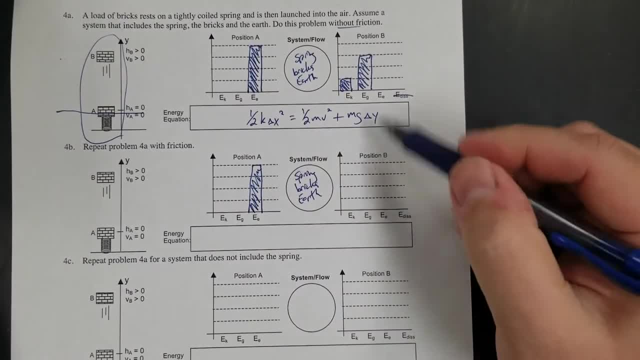 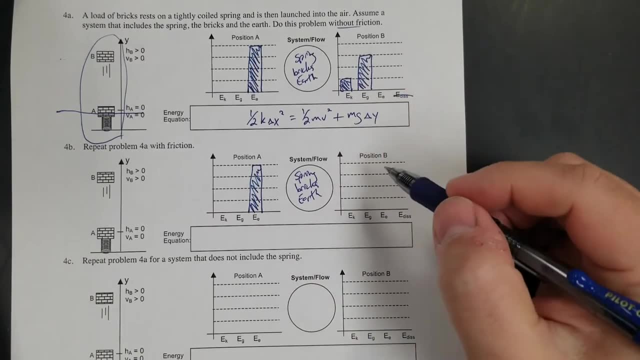 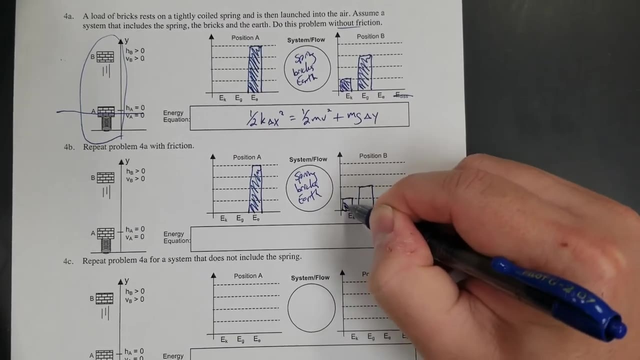 All right. So now there's friction, So that spring when it lets go it's going to produce some thermal energy, right? Because the molecule is moving around in the spring. So I'll take that out of the gravitational. So kinetic gravitational, and I got to have a block of heat. 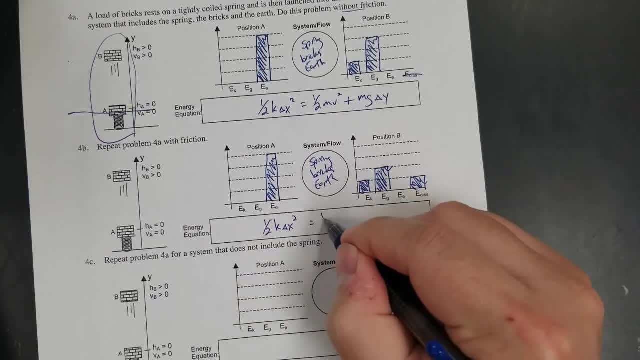 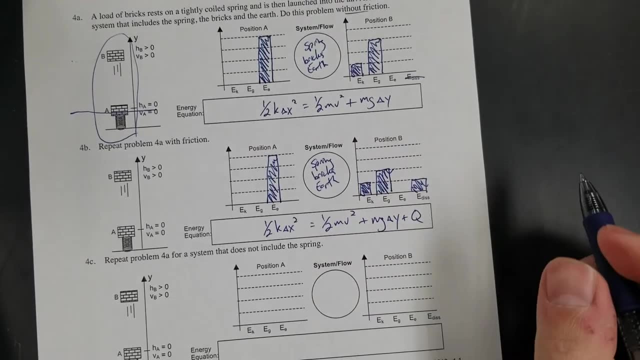 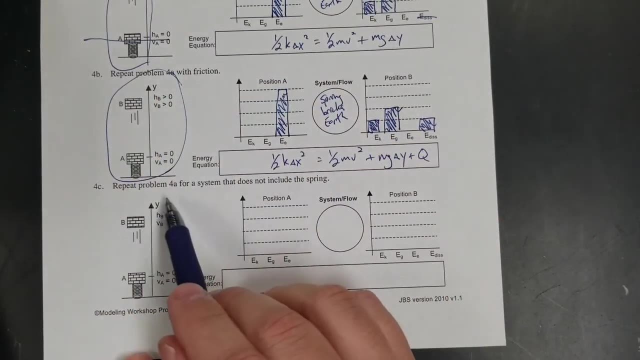 So one half kx squared equals one half mv squared plus mg, delta y Plus q. Okay, All right, So let's do this one Repeat. So in this one this system was the whole thing right. So this one, I'm changing the system.